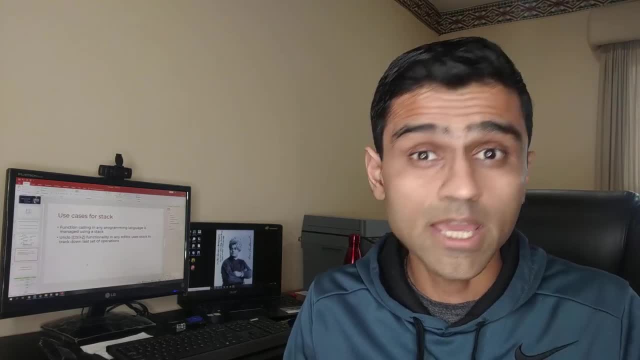 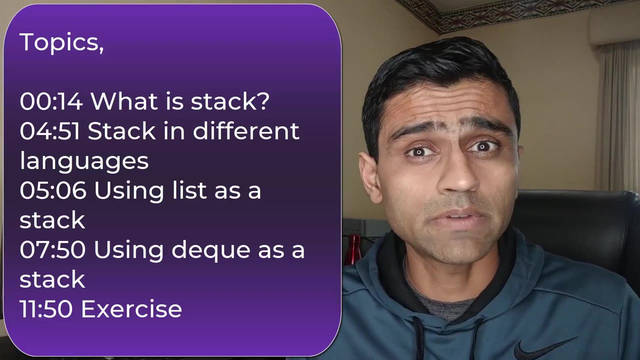 We will be looking at a very important data structure called stack today. Here is a list of topics. As usual, we will go over some theory first, then implement stack in python and in the end, we have very important exercises for you to solve. First, I want to show you a use. 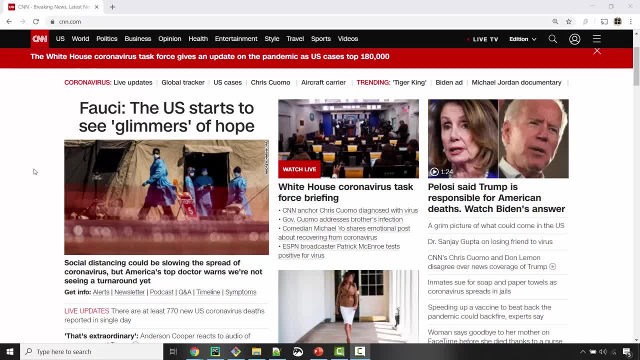 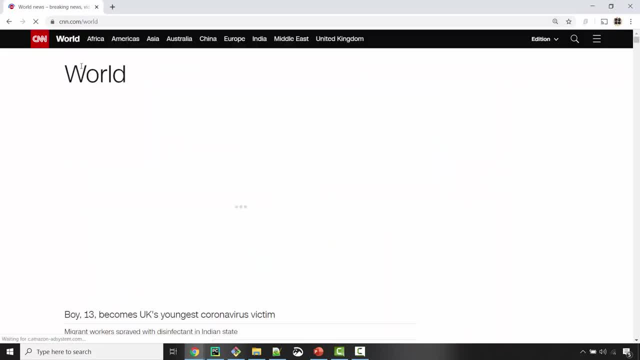 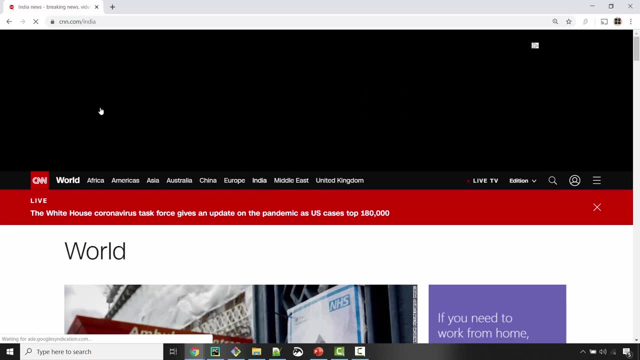 case where using stack data structure could be beneficial. I'm on this website and on this website I can navigate through various pages. Let's say I'm reading world news news, then I want to read news in India, then I want to read news in China. Now, when I go through all these, 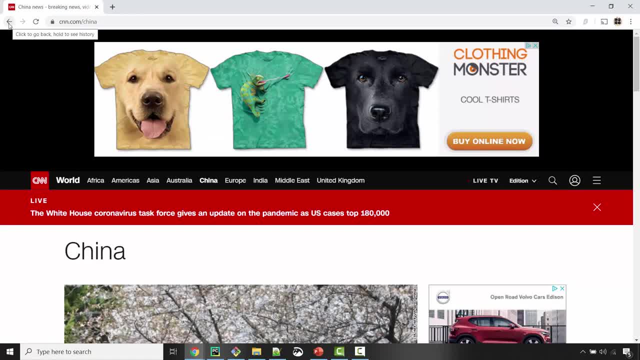 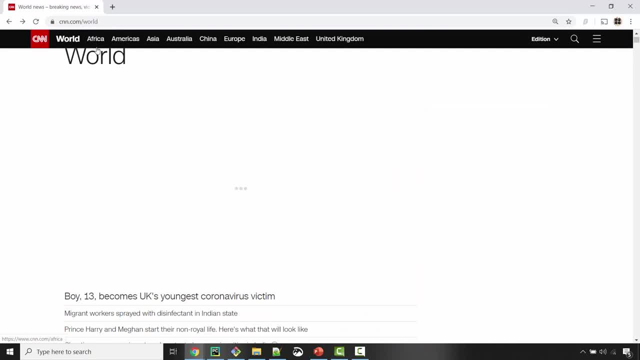 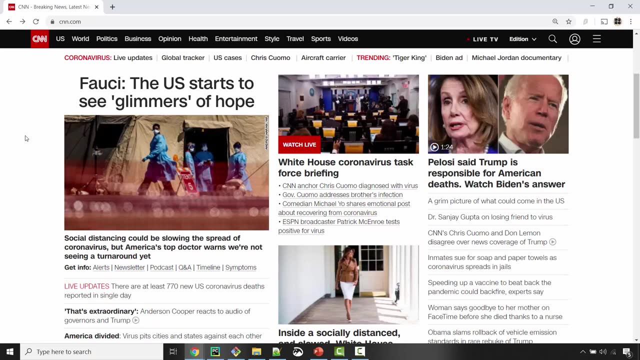 pages. the browser maintains history of it and when I press back button, it will show me the last page that I visited. See, I visited India, before that I visited the world page and before that I was on a home page. So just imagine if you are a browser developer. how would you manage this history in terms of data structure? 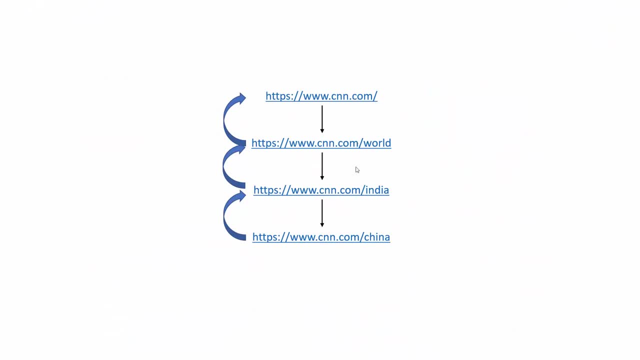 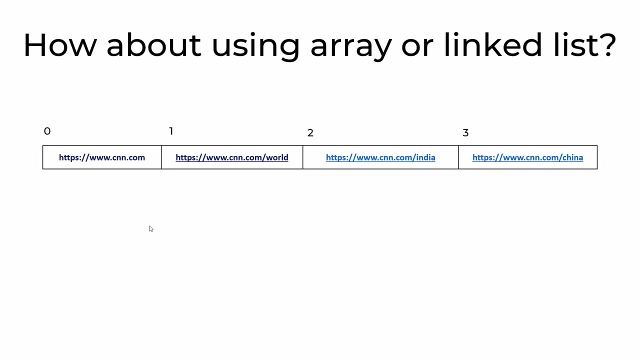 This is a pictorial representation of links that I visited in this order, and when I click on back button, really I'm going to the last page that I visited. Okay, so I am now traversing these links in a backward order. One option I have is I can use maybe an array to store all these links and 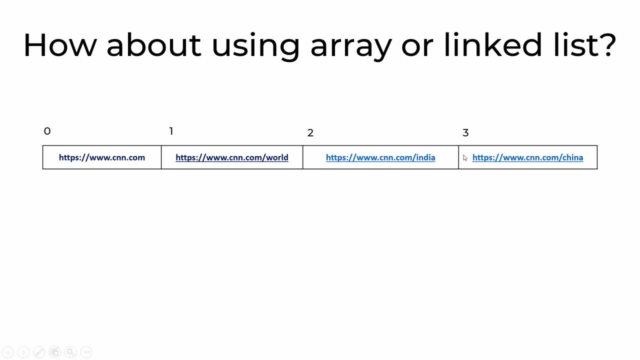 whenever I want to get the last element, I have to go to the end of the array and pop that element out. Another option is, of course, you can use link list. but the issue with these two data structure is that, for example, if you are using 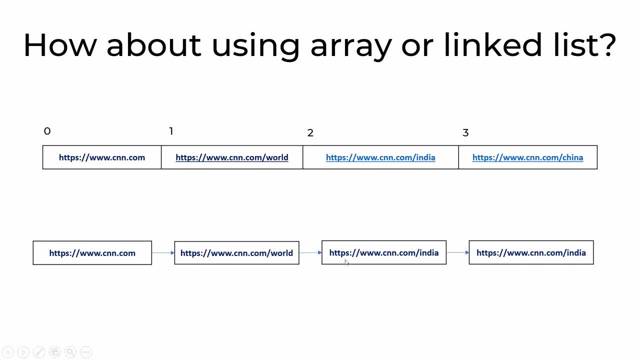 link list. you have to traverse the link list to go to the end and that end will give you the last link that you visited. So every time you are doing order of an operation. similarly with the array, the problem is you have to use dynamic array because you can't use static array, because it can just keep. 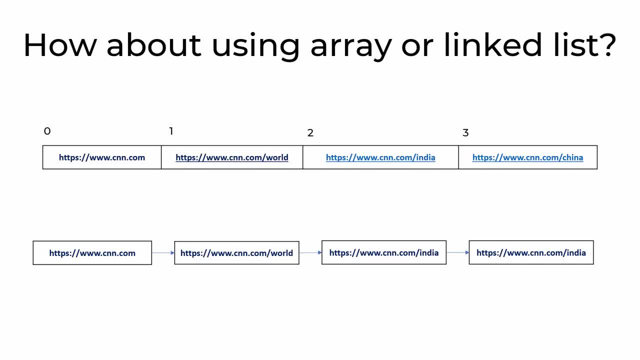 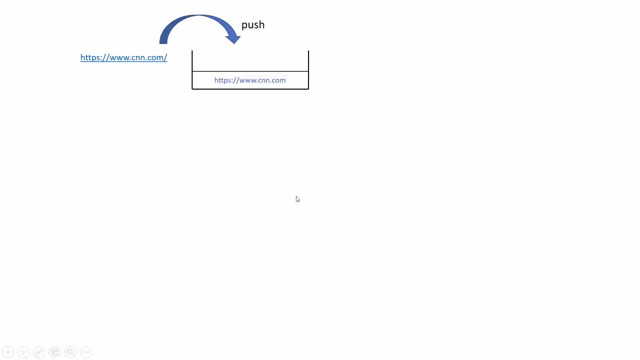 on growing. Also, with dynamic array, there are issues such as memory relocation and copying the elements, etc. In this situation, imagine you have a data structure like this, where once you visit a link, you keep on pushing the elements to that particular data structure and then, when user. 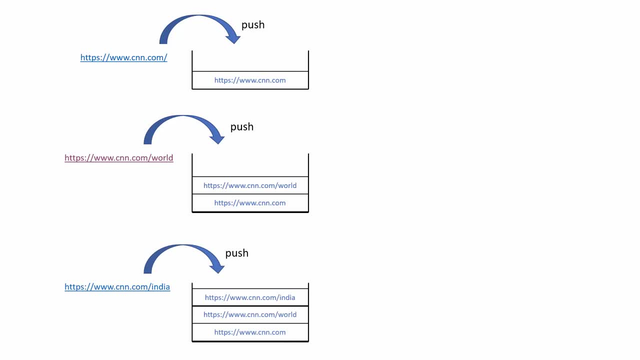 clicks on back button, you retrieve the last element that you pushed. Okay, so there are push operation and the pop operation will pop out the last element. so here you are doing last in first out operation, also known as li fo, and this data structure is called stack. okay, stack is a last. 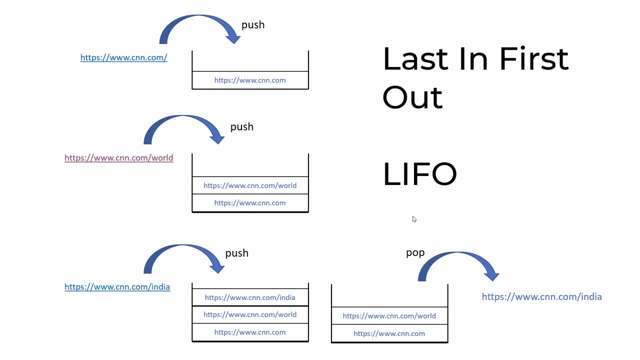 in first out data structure where you keep on pushing the elements and when you say pop, it will pop out the last element that you pushed. if you have a stack of dishes in your kitchen right when you are washing the dishes, when you create a stack when you try to remove the dish, 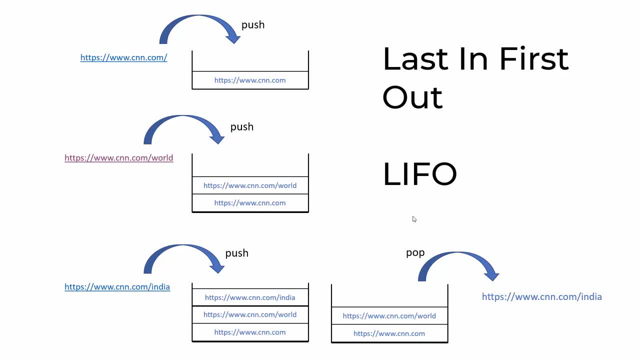 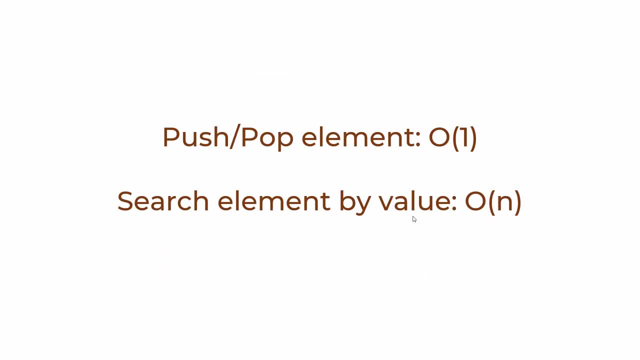 from the stack. you will be picking up the last dish that you pushed on the stack. okay, so stack is exactly that data structure. pushing and popping element is order of one or a constant time operation. if you want to search an element in the stack by a value, it will be order of n. bigger complexity because 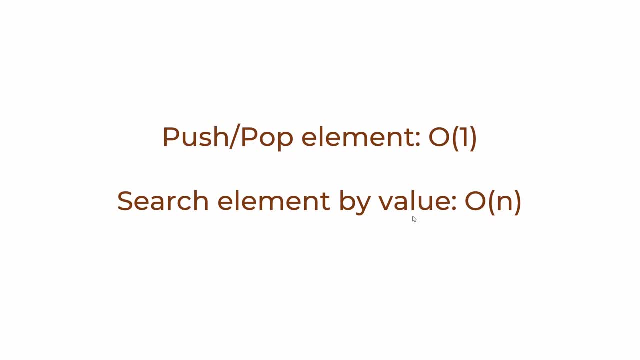 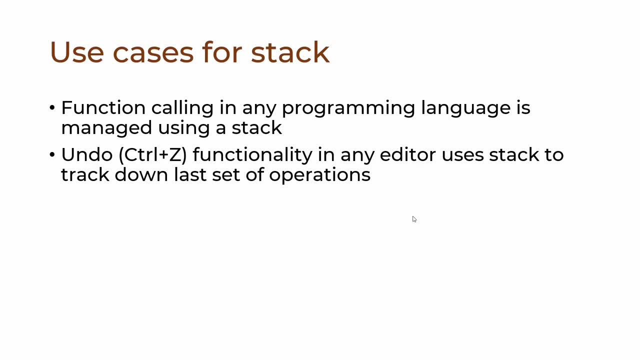 you have to go through each of the elements and you have to locate that particular element. some of the use cases for stack is in any programming language language. when you are calling a function and then that function calls some other function internally, compiler will use stack to push all those functions to maintain the order of those functions. basically, in any 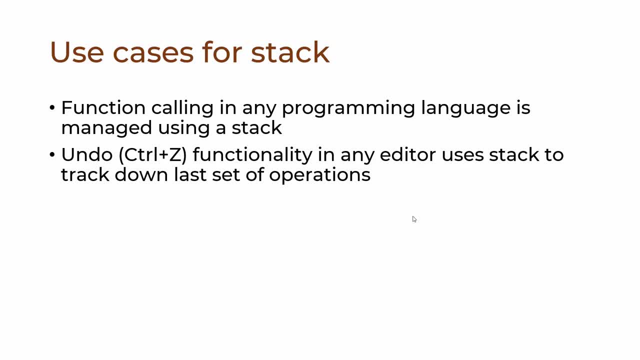 additional function. you have to search an element in the stack by a value. it will be order of n later. let's say you have microsoft paint or word or microsoft excel. they have this undo functionality. so undo functionality will undo the last operation. for that also they use the stack i mentioned. 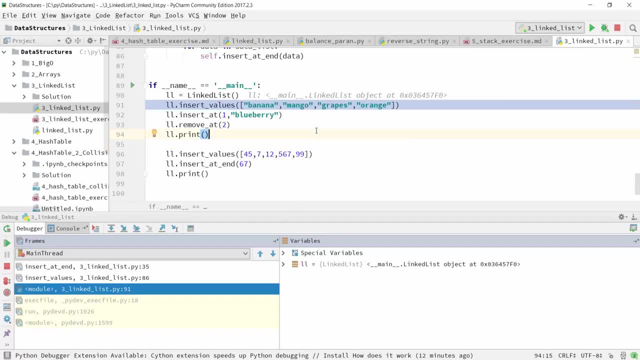 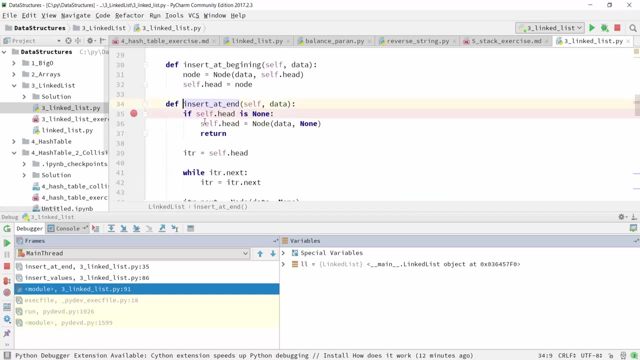 that compiler or programming language uses stack in underneath. so here i want to show you one example where, see in this code, i am calling this function called insert values and insert value function will eventually call insert at the end. so when i put a break point here, it will see it will stop. 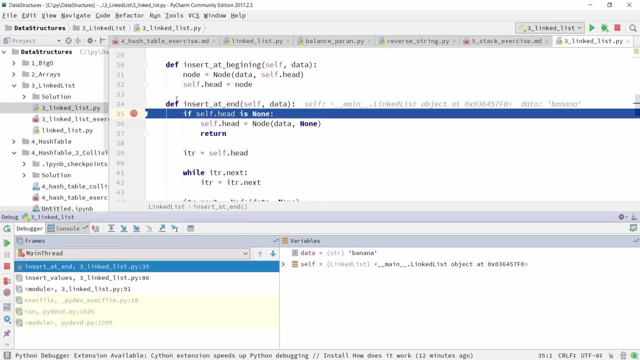 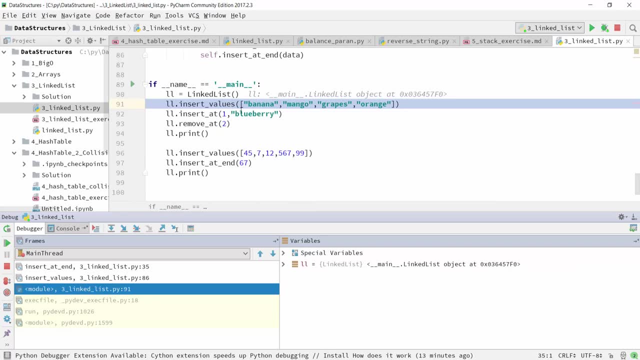 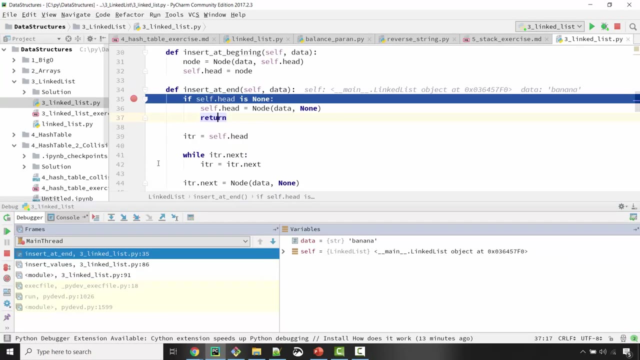 here. but the call for insert at n came from insert values and insert values came from this main function. so this particular thing that you are seeing here is called the function stack. basically, function is calling it one by one. you can do F10 or just press this button and you'll realize that. 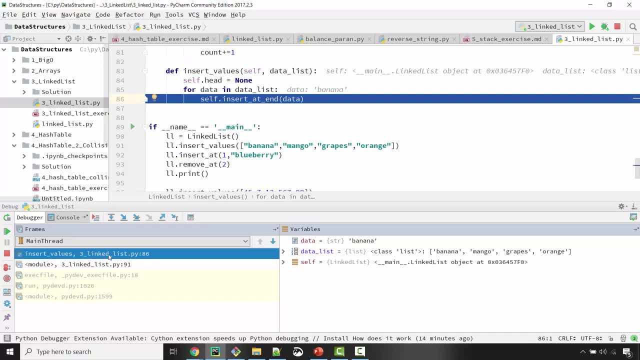 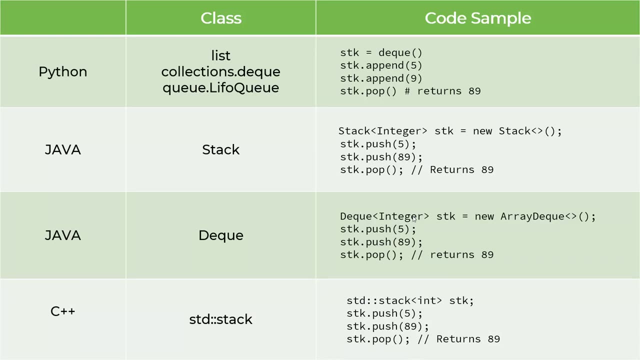 it comes back. see, now i have two functions, so it will just go to the last function function that you call. so this is the standard example of how stack can be used in programming languages to manage the function calls. here is the stack implementation in different programming languages: python: in python you can implement stack using list, collectiondq or li4q. java: 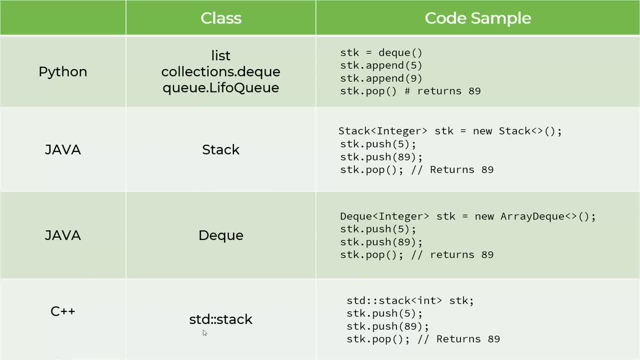 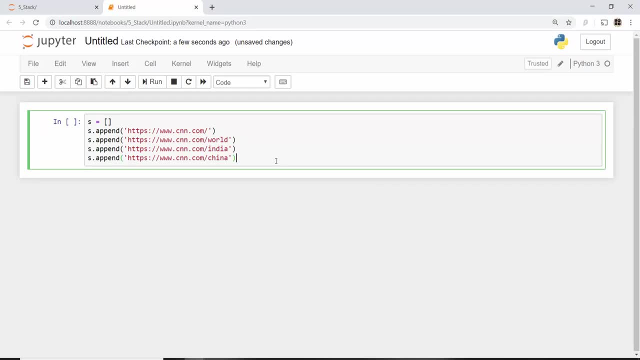 also has multiple classes and c++ has std stack. now i'm going to show you how you would manage the browser history back functionality using a list in python, so the python list can be used as a stack here. i have created this list and appended all those web links that i visited. okay, 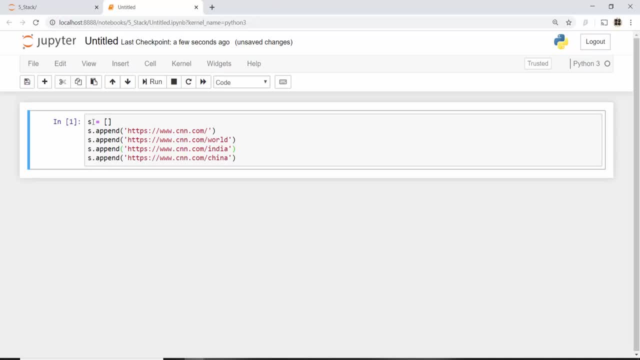 and when you do ctrl enter, it's gonna create the list and append all these links. now, when you want to get the last thing that you appended, you can call pop function and pop will give you the last link that you visited, which was cnncom slash china. and now, when i look at s, 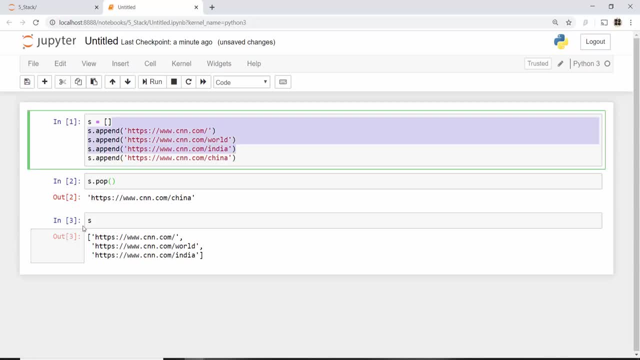 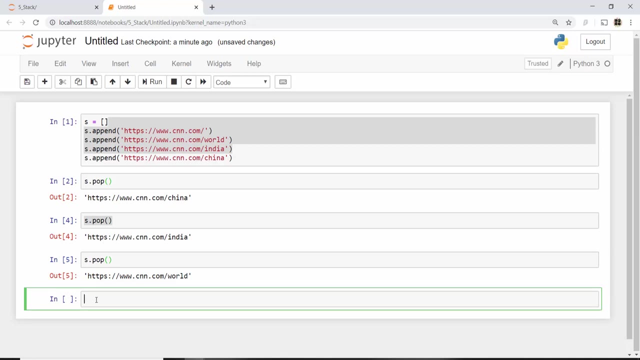 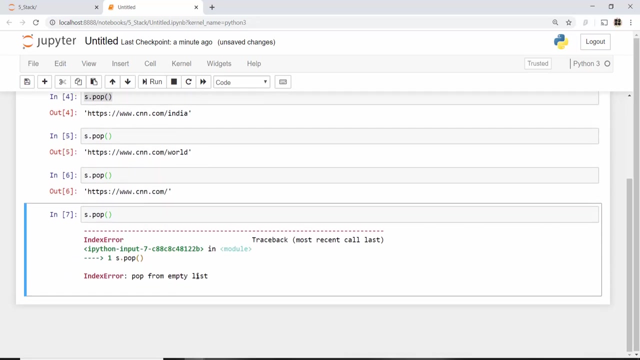 it will have only three things, you see, and you can then call pop again. so that gives you india pop again, okay world. then pop again cnncom, and when you do cnncom pop after that it will say that you cannot pop from an empty list. so the pop operation in stack. 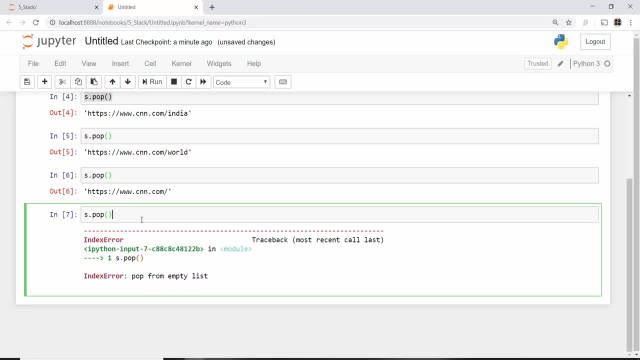 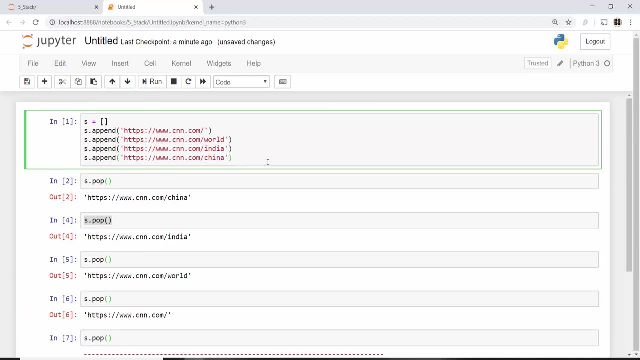 will pop out the last element. it will return the last element. it will remove the element from the list. now, if you don't want to remove the element from the list, so let me execute this once again. okay, let's say i don't want to remove the element from the list, but i just want to get the element. 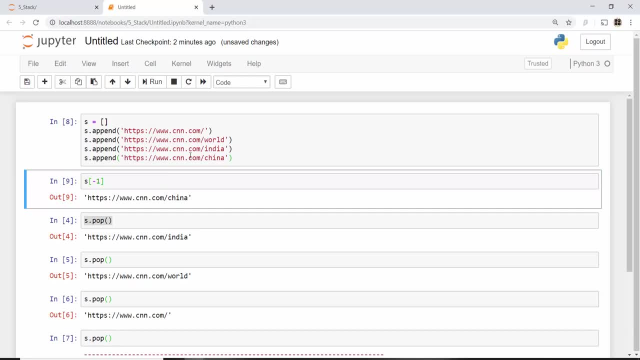 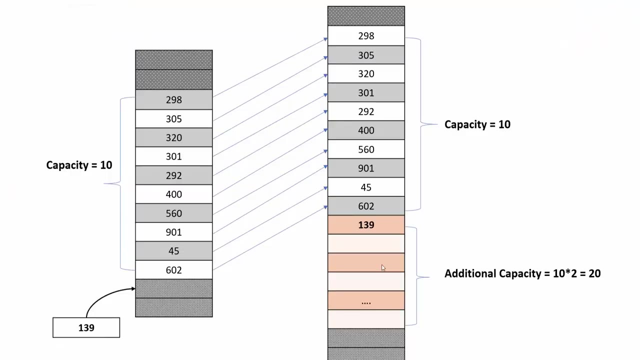 so in python you know that you can use minus index to get the last element. so if when you say minus one, you get china back and your list is still not changed, while you can use list as a stack in python, the problem with list is that it is a dynamic array. for example, if you have a list, 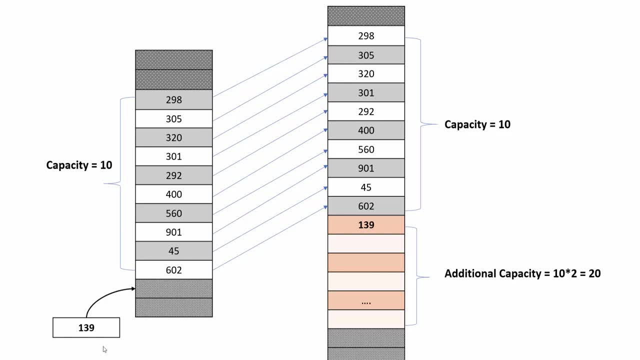 with a capacity of 10, let's say, and if you want to insert 11th element internally, since it is a dynamic array, you can должен to insert it as a stack. and if you want to insert it as a stack, you can array what it's gonna do. is it now see? in this case it doesn't have the capacity for 11th element. 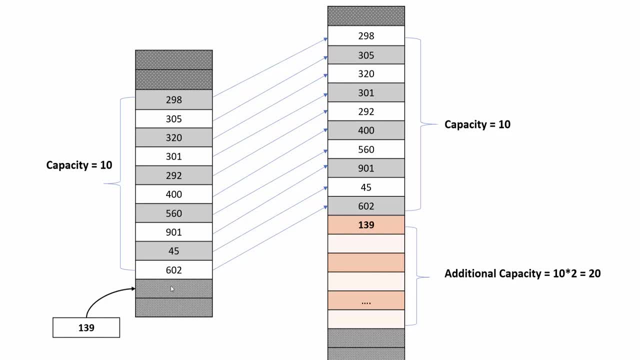 so it will go into some other memory area, it will allocate some extra capacity. usually if your current capacity is 10, it will allocate the current capacity into two- those much additional memory location- and then it will copy all those 10 elements here and then now it will insert this: 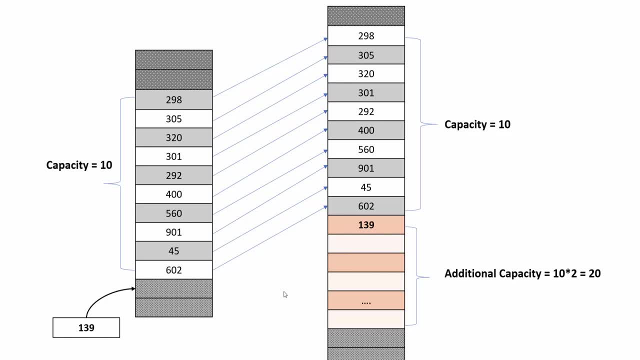 139. so the problem here is not only it has to allocate new memory, it needs to copy all existing elements. if you have million elements, you have to copy all the million elements, which might be costly. for that reason, using list as a stack in python is not recommended. the recommended approach: 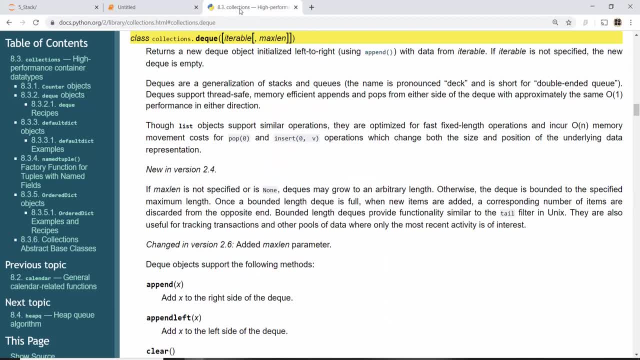 in python is to use collectionsdq. now, if you look at collectiondq documentation, it says that they are a generalization- Generalization of stack and queues- and they are implemented using doubly linked list. So you don't have to worry about The issues that you face with dynamic arrays. Okay, it will. 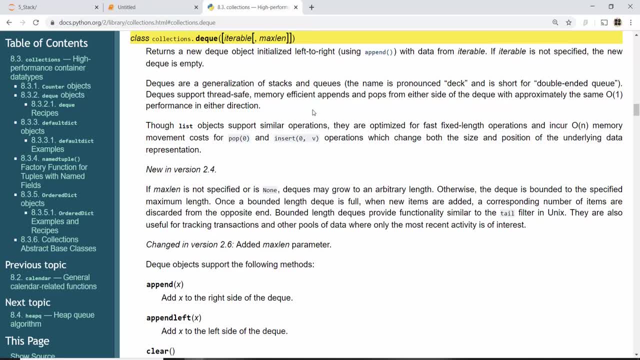 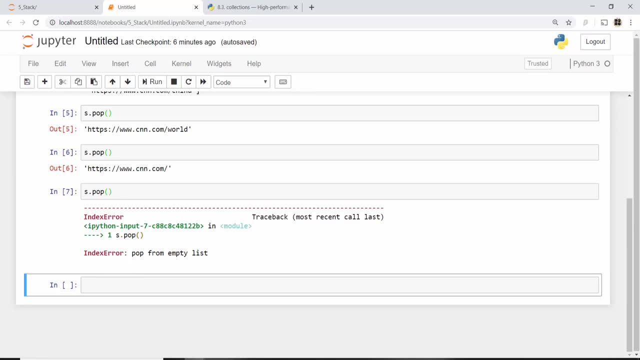 Allocate new location as and when needed, and you don't have to worry about copying the current elements into the new memory location. So let's implement stack using DQ now. First thing you have to do is you have to import DQ from collections. Okay, so I'm gonna do. 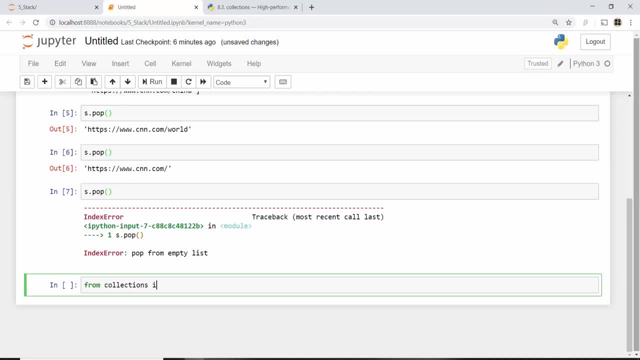 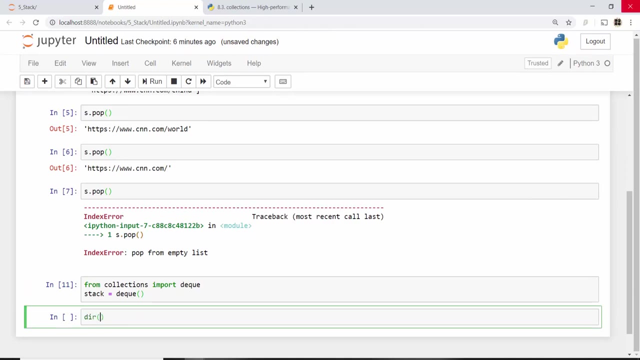 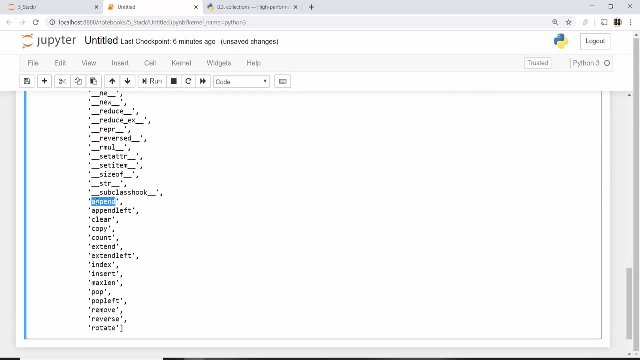 from collections, import DQ and then my stack is a DQ. Now I want to see what type of Method this has. so when you do dir stack, it will show you all the methods. So I see methods such as append, append left And so on. you can also refer to the documentation. 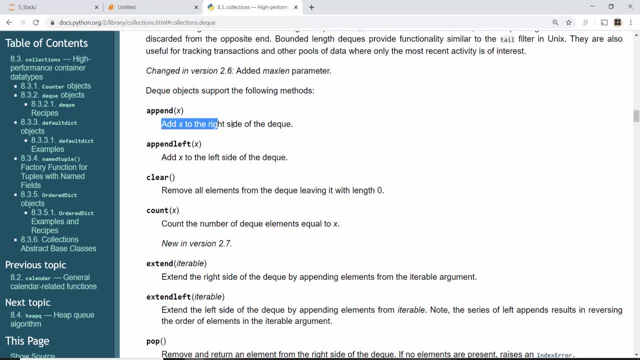 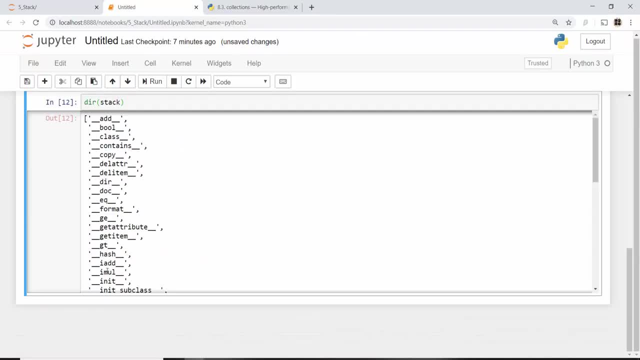 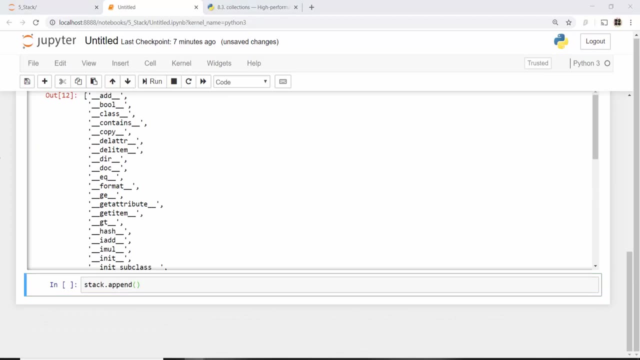 Okay, so here it says: append will add X to the right side of the DQ, and that's what we want. We don't want to use any of this left function. Okay, so let's do stack dot append. and In here I Want to append the link that I visited. 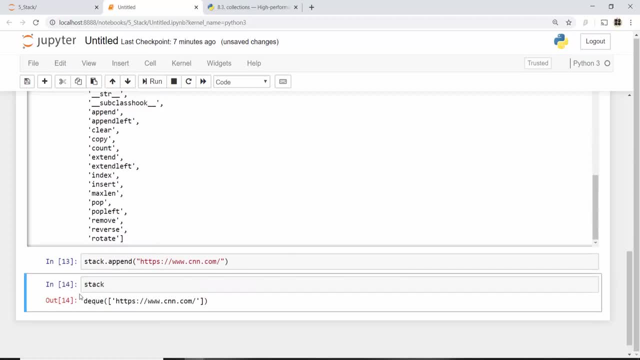 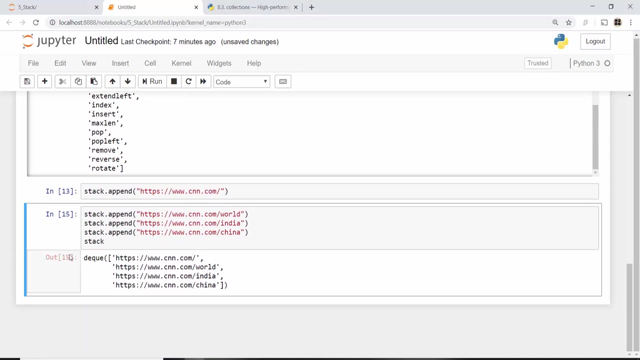 Let's see how the stack looks like. see, stack has this. now you can append few more things, so I am just going to append this one and the other two links that I visited while browsing. see, it creates a DQ like this and when you do stack dot pop, it will obviously return. 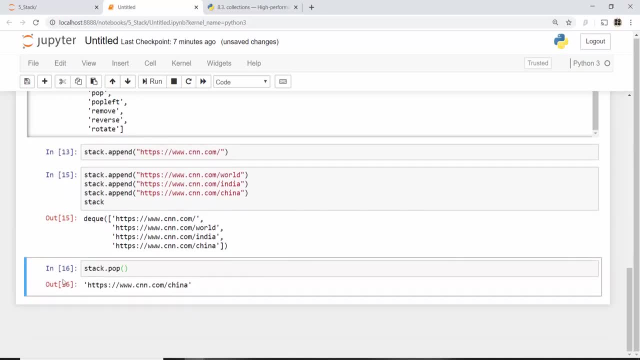 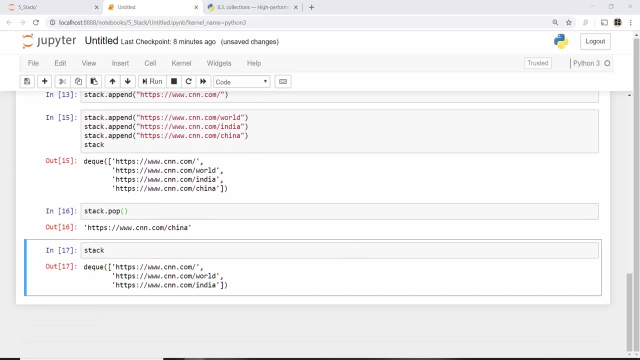 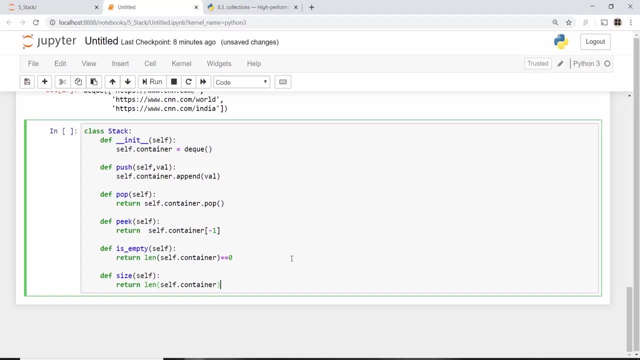 you the last element, and not only it returns the last element, it will remove it. so now cnncom slash China is not in my stack anymore. now here I created a stack class just for fun, using DQ. you can use DQ, as it is for a stack class. 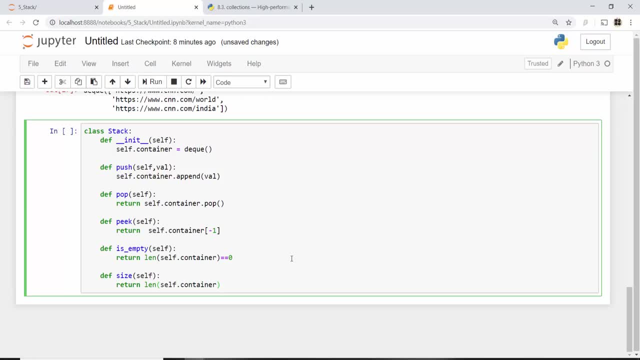 but I want to follow the proper stack prototype and use the functions such as push, pop, peak, etc. that's why I created this class. it looks pretty good, so I am just going to do that. and I am just going to do that, and that's why I created this class. it looks pretty good, so I am just going to. 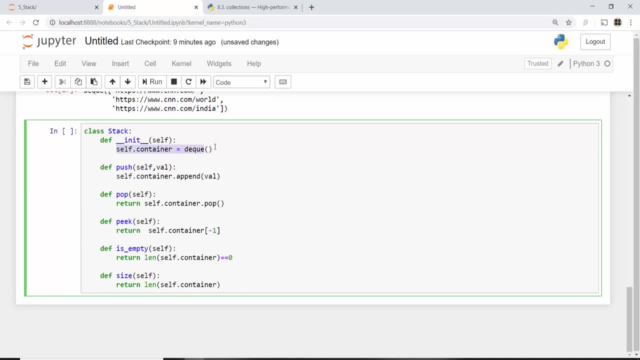 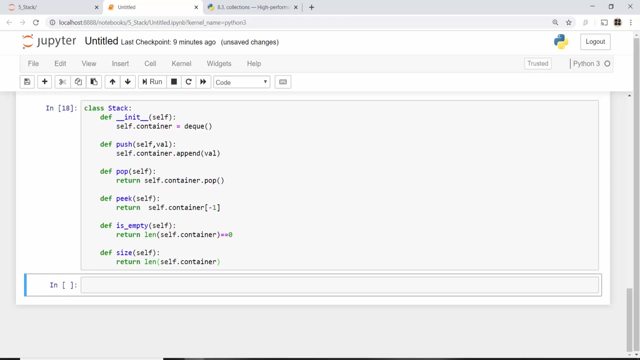 pretty simple. internally, I have a container which is nothing but an object of DQ class. when you do push, I am doing append to the push. all right, so you can look at all these methods. these are like very, very simple methods. this is my Python implementation of stack class, and now I am going to try a few things with 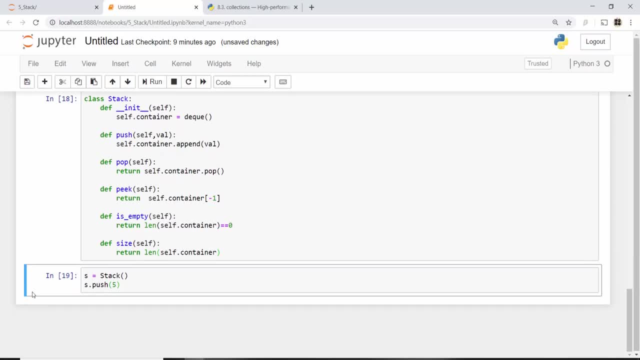 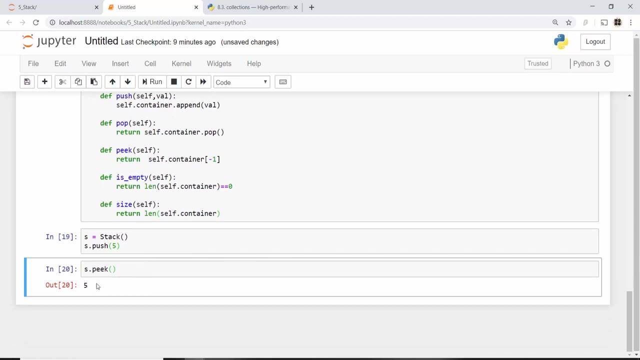 this stack class, right. so I pushed five element five here and then I'm gonna call s dot peak. so s dot peak will return 5, but it will not remove 5 from my stack. okay, so I still have value five. so if I call, you, call s dot peak once again, it will still return me 5 if I do. 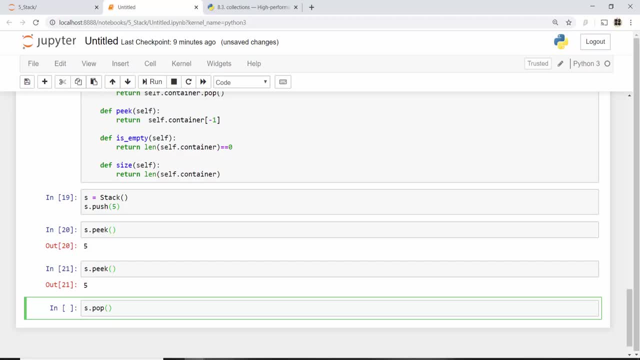 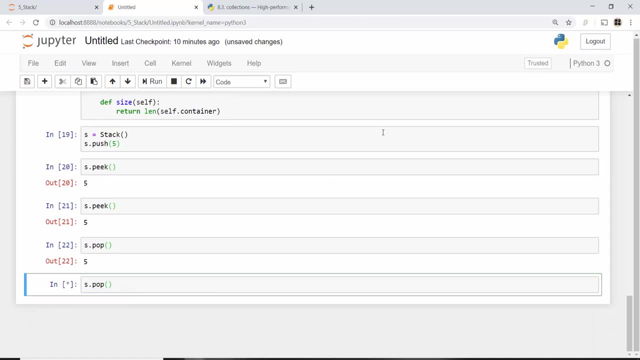 s dot. this is: if I do s dot, it will go away ones soon enough. it will still echo when I now do each int that. so this here, sorry ant skills, because I want to pull from the along, which is a different one, and I'm not going to take these. and then I'm 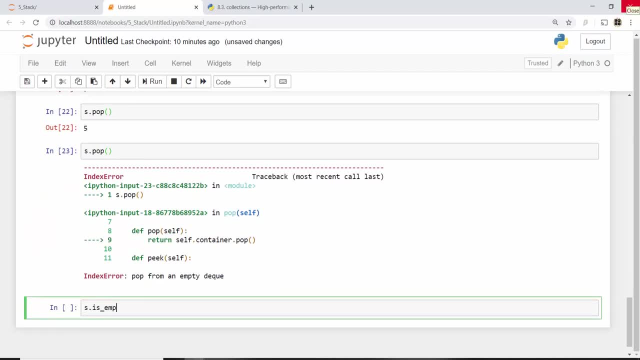 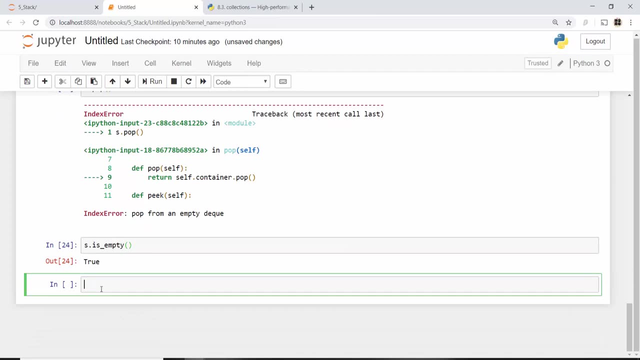 when I call s dot is empty method, it will tell me the stack is. the stack is empty. you can also do s dot push couple of values. so I'm gonna push, let's say, three values, okay, and when you do s dot size, it will return me the size of the. 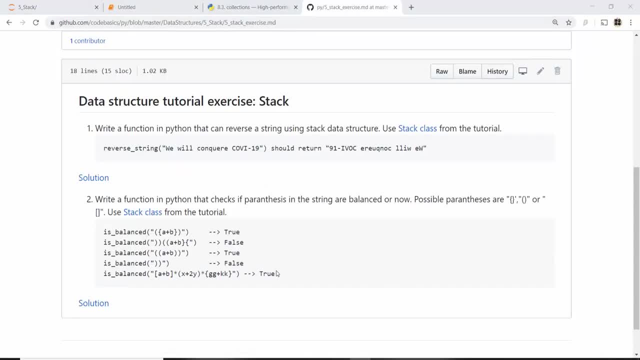 stack. that's all I had for this tutorial. now the most interesting part of this tutorial, which is an exercise. so I have these exercises for you. I have a solution link, but you're not going to click on that link until you solve this exercise on your own, without solving the thing on your own. if you click on the, 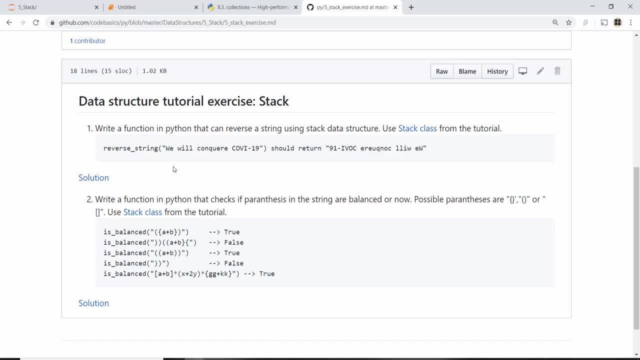 solution link. it is going to download kovat 19 virus on your computer. okay, so be very careful. I have that automation in place so you try things out on your own for yourself. so I'm going to show you how to do that. so I'm going to show you. 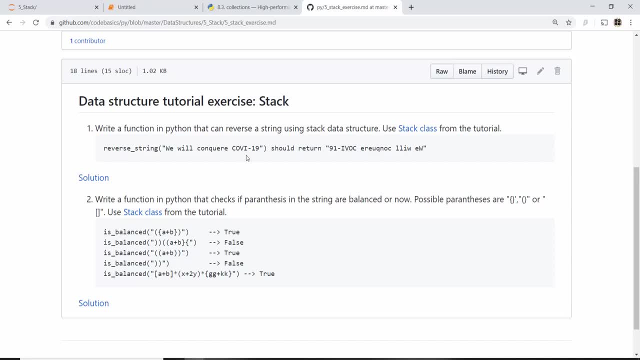 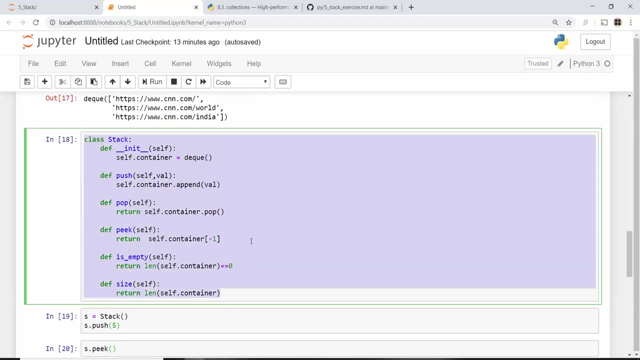 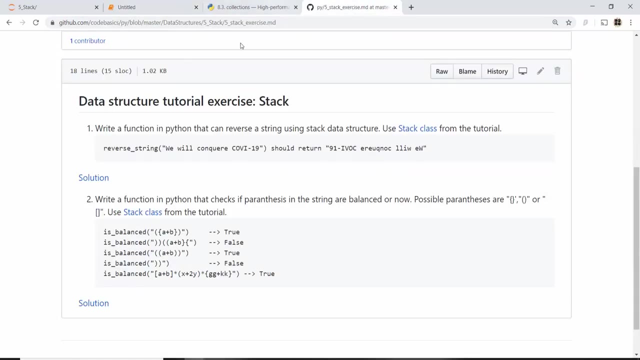 first, then only you look at the solution for the exercises. you will be using this particular stack class that we did in our tutorial and I'm going to post a link of this tutorial, this notebook, as well as the exercise description etc. in the video description. so make sure you check the video. 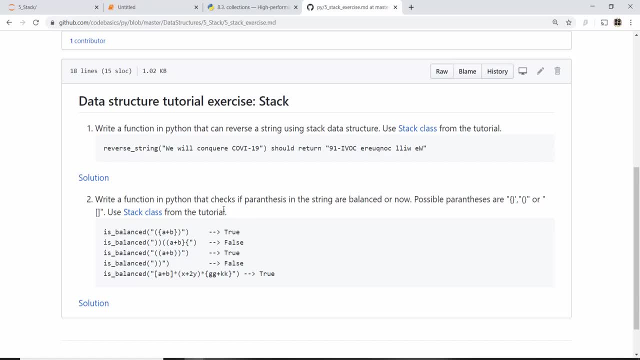 description: work on the exercise also. watch my rest of the data structure tutorials. data structures: as I have said in the минitrack- i work on the exercise also. watch my rest of the data structure tutorials. data structures, as I have said before, are very important in programming interviews, even if you want to become data